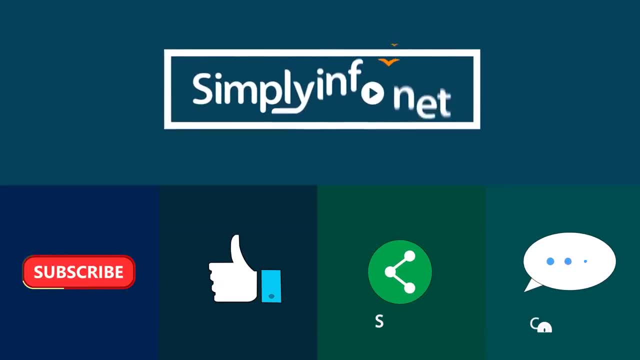 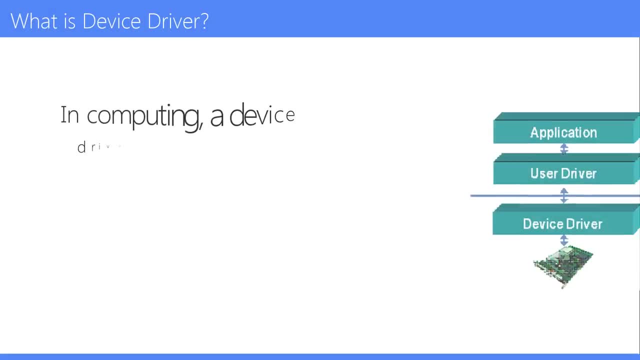 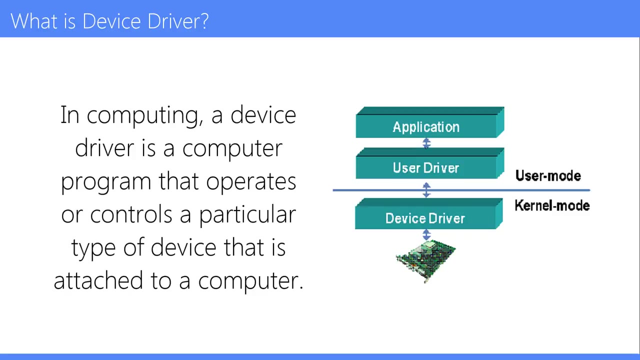 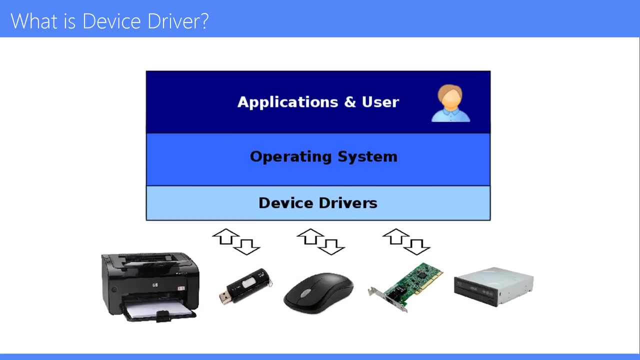 What is Device Driver? In computing, a device driver is a computer program that operates or controls a particular type of device that is attached to a computer. A driver provides a software interface to hardware devices, enabling operating systems and other computer programs to access hardware. 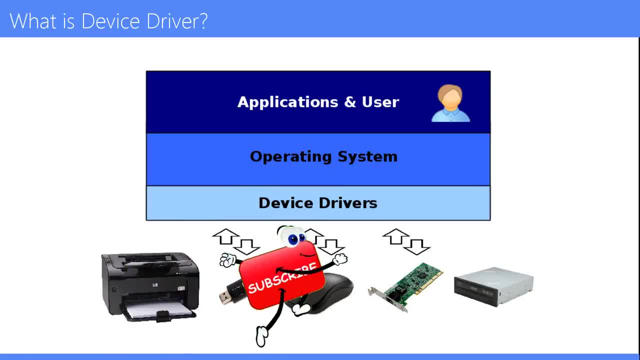 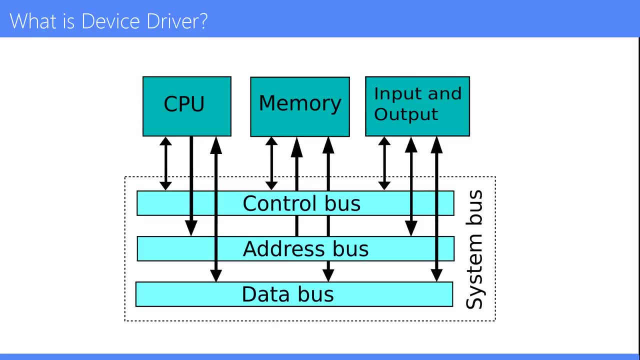 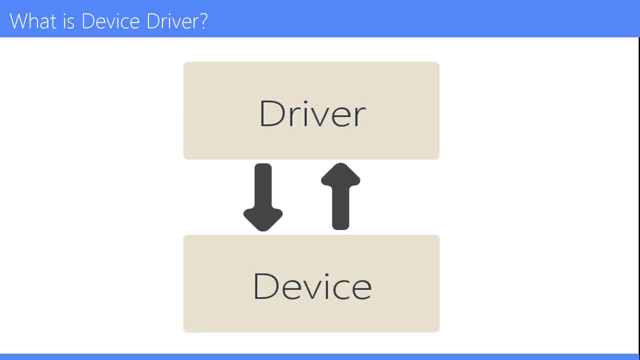 functions without needing to know the precise details of the hardware being used. A driver communicates with the device through the computer bus or communicates subsystems to which the hardware connects. When a calling program invokes routine in the driver, the driver issues commands to the device Once the device sends data back to the driver. 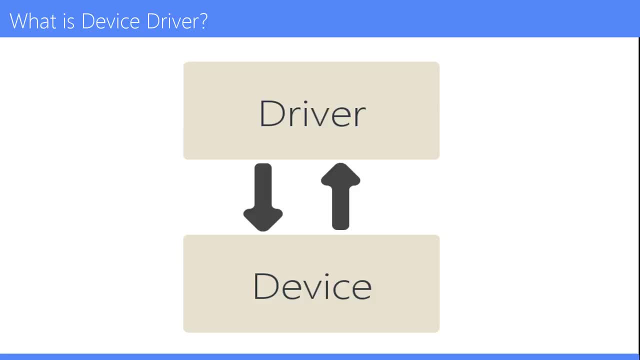 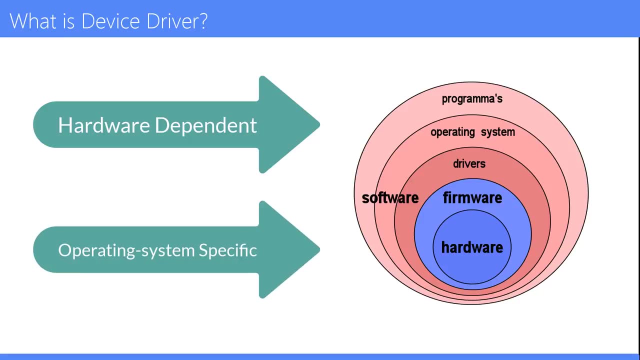 the driver may invoke routineness in the original calling program. Drivers are hardware-dependent and operating system-specific. They usually provide the interrupt handling required for any necessary asynchronous time-dependent hardware interface. For example, a high-level application for interacting with a serial port may simply. 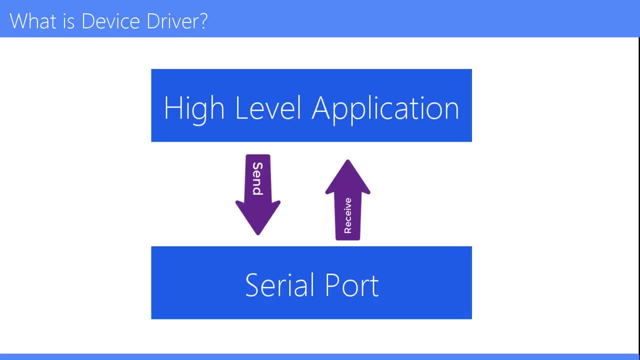 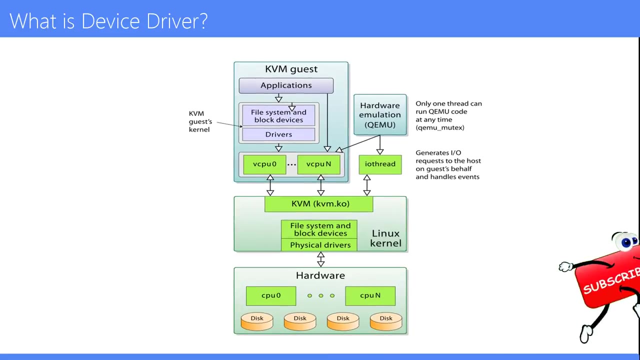 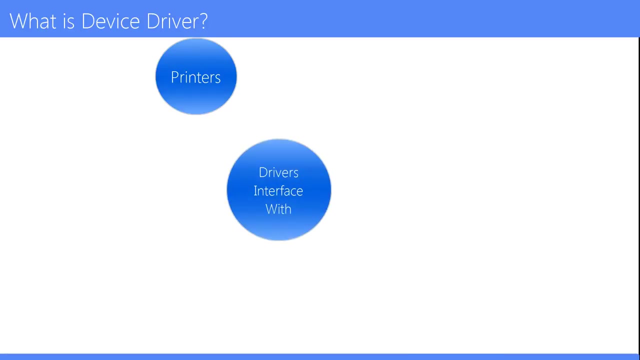 have two functions for send data and receive data At a lower level. the device driver implementing these functions would communicate to the particular serial port controller installed on a user's computer. In modern hardware and operating system, drivers operate in many different environments. Driver may interface with printers, video adapters, network cards, sound cards, local. 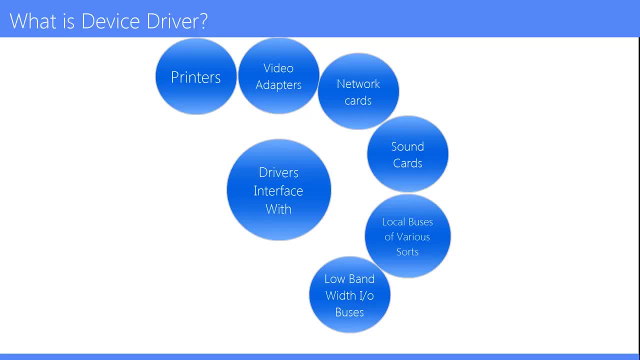 buses of various sorts: low bandwidth IO buses, computer storage devices such as hard disk, CD-ROM and floppy disk. buses via ATA, SAT and other devices. Driver may also be able to send data back to the driver via ATA or SCSI. 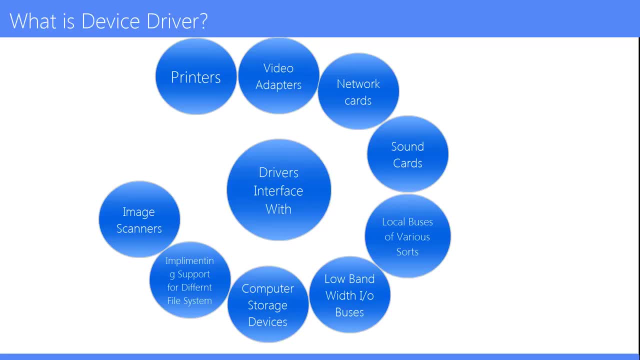 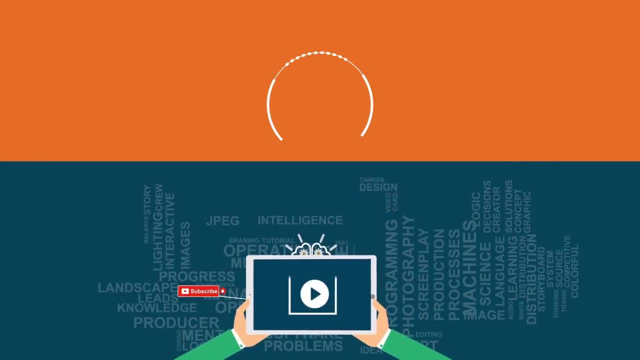 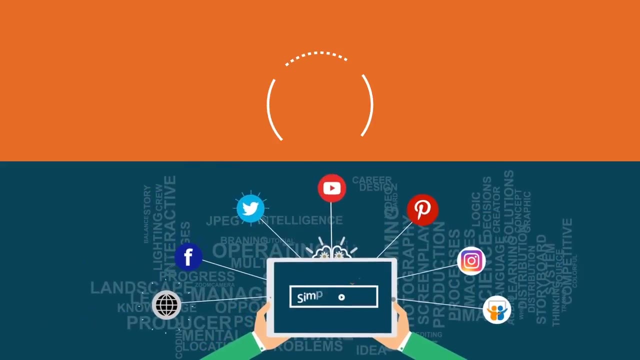 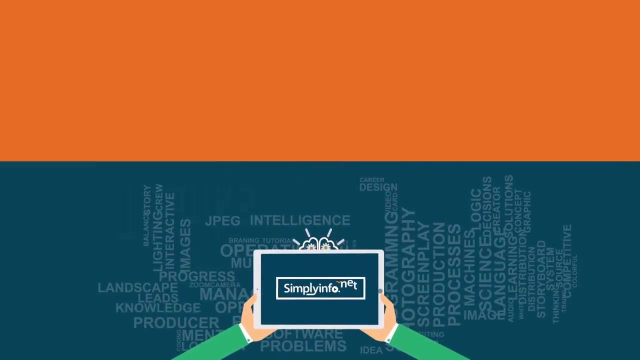 Implementing support for different file systems, image scanners and digital cameras. For more information, please visit http//wwwhamskeycom. http//wwwhamskeycom.